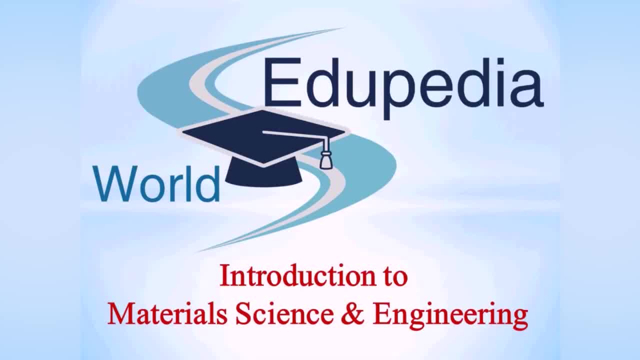 Hi everyone. welcome back to the course on Introduction to Material Science and Engineering offered by Edipedia World. Previous lectures I introduced you to the concept of crystalline materials and amorphous materials and how there is a long range ordering in crystalline materials. 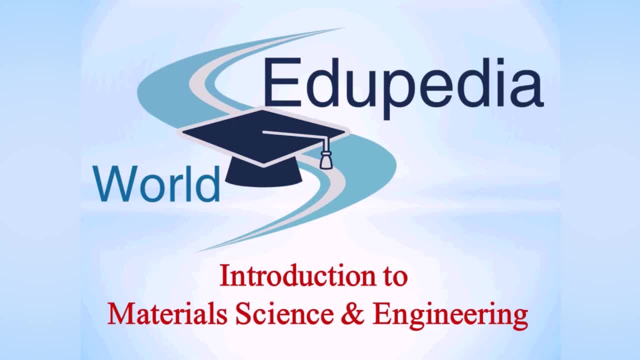 Now, with this idea, you might think that should a crystalline material have order throughout the material or in a part of the material, a part of the specimen? So this is the exact question which I addressed in the previous lecture, in which I showed you the difference between single crystal and polycrystal. 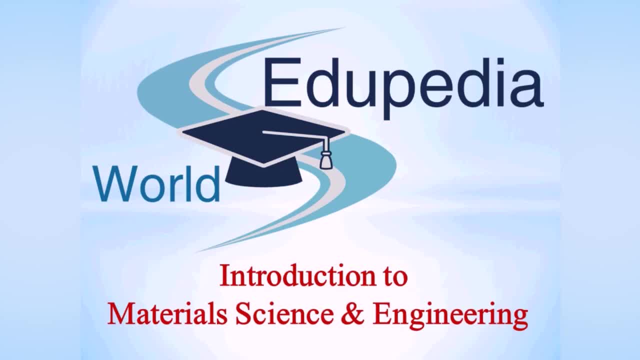 A single crystal is one where there is the complete specimen, has order throughout the specimen, Whereas a polycrystal has different crystals throughout the specimen. But now imagine you have, even if you have a single crystal or if you have a polycrystal, then is it possible that there is an uniformity within the material, or is it that even for a single crystal or for a polycrystal, there has to be exact ordering throughout the material? 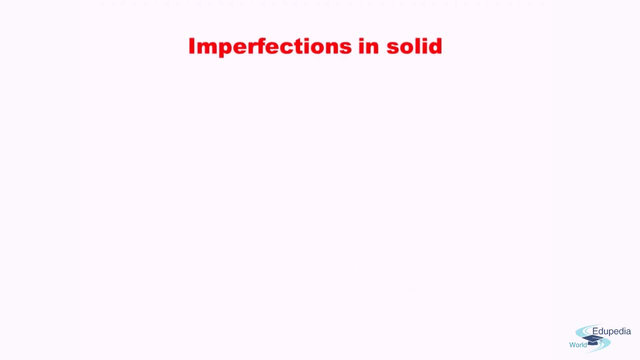 What I mean is that all the atoms Should be at exact position. no atom should be missing from anywhere. no additional atom should be anywhere. Is that the case? As we'll see in today's lecture, that is not the case, So our discussion will be on imperfections in solid. 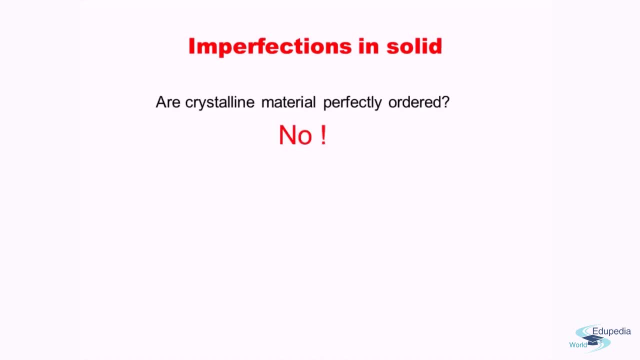 The case we have studied till now are perfect solids. Are crystalline materials perfectly ordered? That is the question. And, as I said, no. So if the crystalline materials, No, If it's not perfectly ordered, then what is the exact scenario? 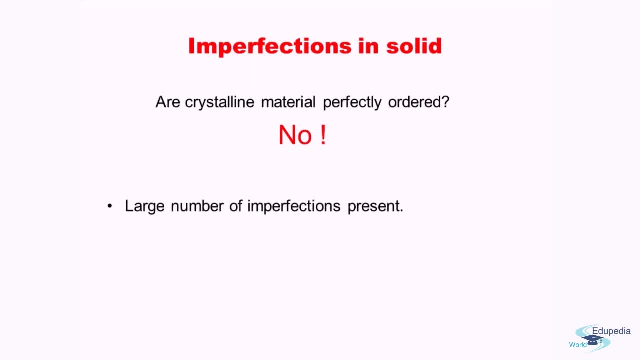 What is the practical scenario? There are actually a large number of imperfections present in any crystalline material, be it single crystal, be it polycrystals. There, the type of imperfection present may be different in single crystal and polycrystalline material, as we'll see. 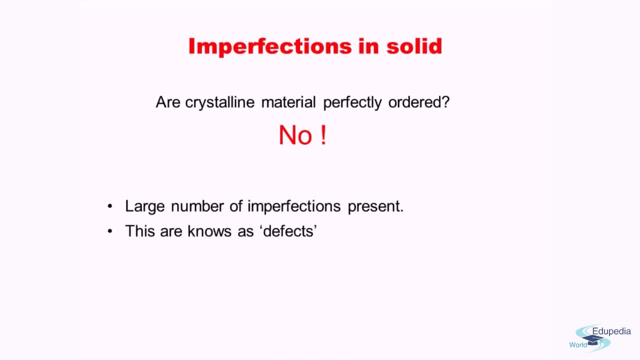 And also within the polycrystalline material, there may be different kind of imperfection. The meaning of the term is different, So this particular kind of imperfections which are present in a crystalline material are known as defects. 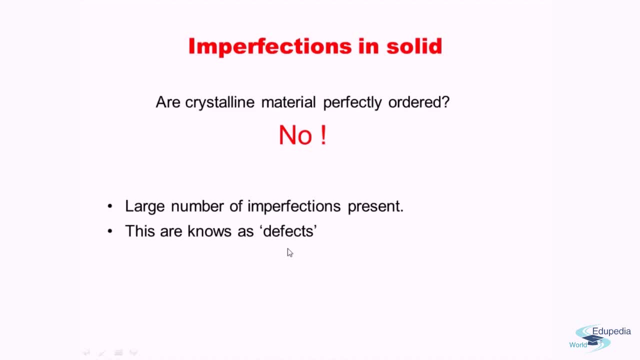 So, as the term suggests, defect is kind of a deviation from a perfection. That's why defects And this defects. You might think that the defects which are there hamper the properties, But as a matter of fact the defects are sometimes very important for property enhancement too, because all the applications 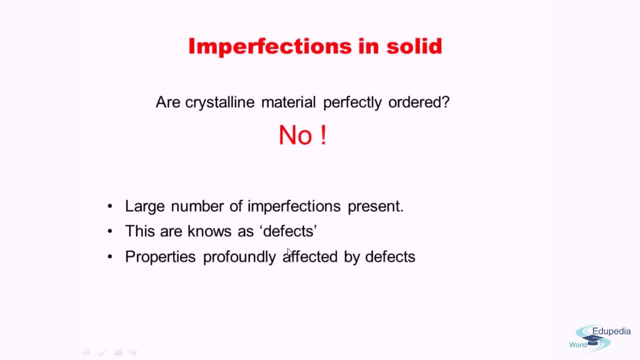 have different requirements and different applications. requirements can be met by tailoring the amount of defect and the types of defect we have in the material. so the properties are profoundly affected by the defects that are present in the material. and defects in crystalline material or lattice is irregularity in one or more dimension. 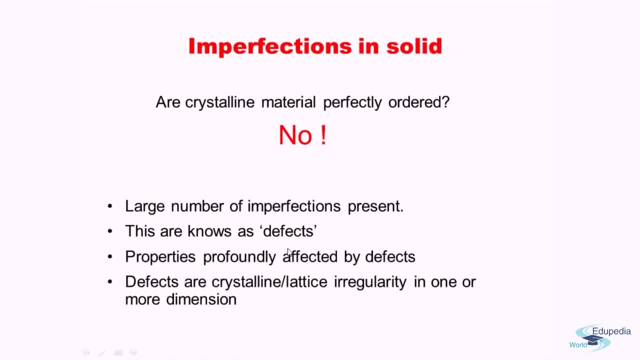 so what this means is that defects can be rather not just one or more dimension, it can even be in zero dimension as well. see, it can even be zero dimension. so crystalline κ lattice irregularity, which is known as imperfections or defects, can be in zero dimension or point. 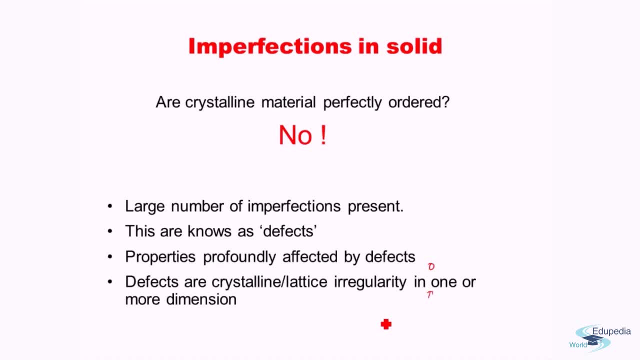 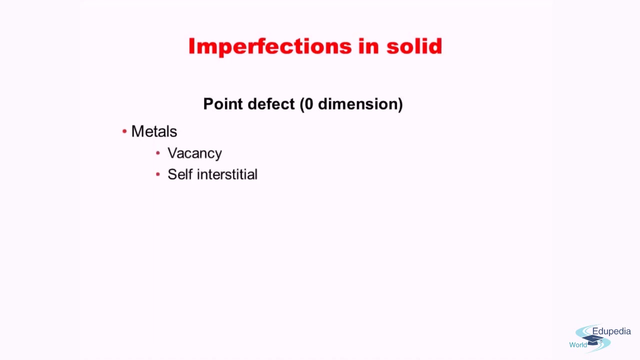 defect: one dimension or line defect, two dimension or surface defect, and three dimensional, or what is known as volume defect. So to begin with our study, let us see what are the point defects that are present in a solid or the zero dimensional defects In metals. we can have either vacancy or self-interstitial. we will see in details about each of the individual. 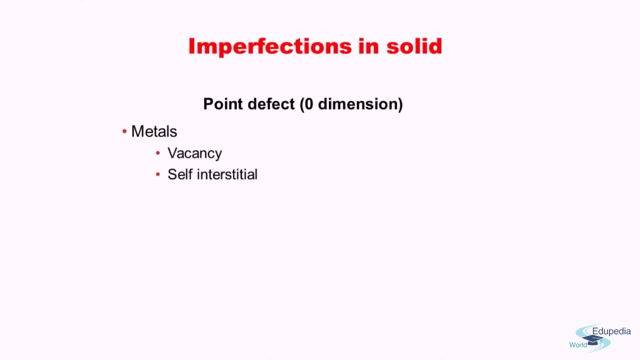 type of defect in the coming lectures, but just to give you a brief glimpse: vacancy means atom is absent where there should be an atom, whereas self-interstitial means extra atom is present in the void between atoms. So this is effectively less than or equal to zero dimension or point defect. 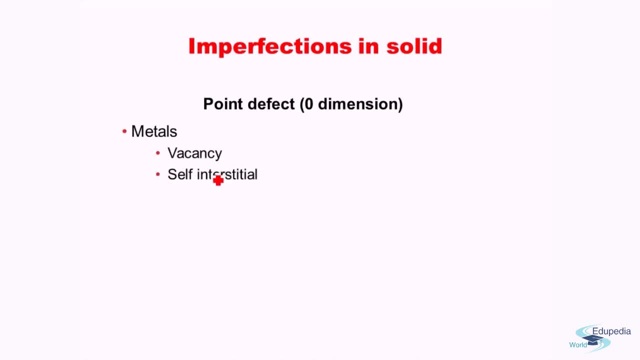 Less atom than there should be. this is effectively more atom than there should be. Then point defects in the case of ceramics can be Frenkel defect and Schottky defect. Frenkel defect is basically atom missing from its location and is located at a different. 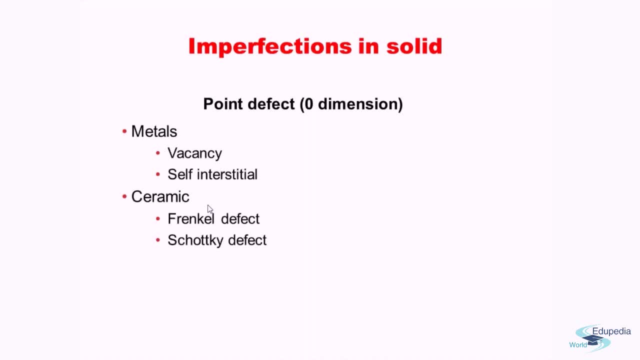 location. Schottky defect is basically two atoms missing. we will see in details later. Then we have impurities That can be both in metal case and ceramic case. Now, what do I mean by impurities? See, the idea is that for a particular metal or for a particular ceramic, the composition, 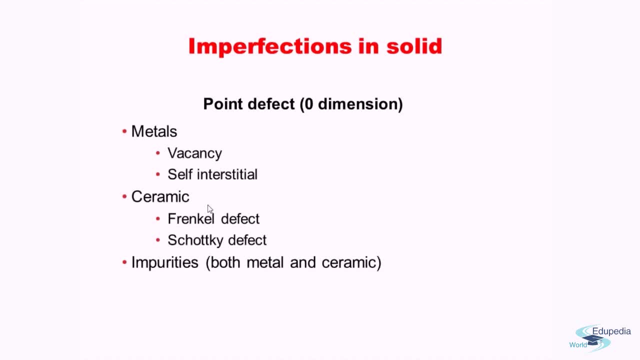 is defined. Let's say, for example, iron. Iron has a few atoms present at its lattice sides, right, But suppose that we add something to iron? let's say we add carbon that makes steel. So in addition to the iron that was initially there, we now have additional element, which. 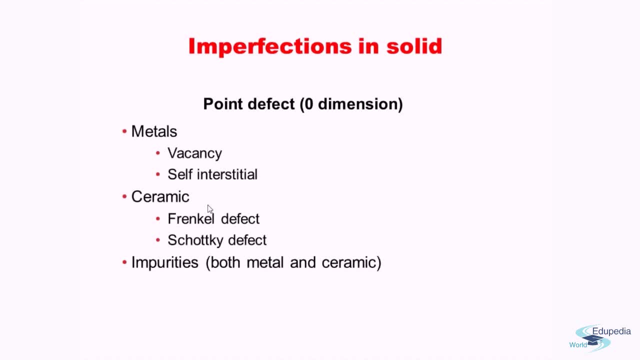 was not supposed to be there. that is carbon. So these thing which is externally added or which is externally present, which should not be there, are known as impurities. right Now the impurities can be present both in the metal case as well as the ceramic case. 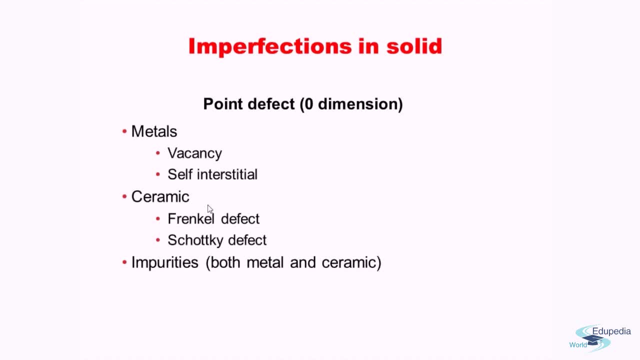 And what are the type of defects that can be under the categorization of impurities? Let's see The type of defect. will be substitutional or interstitial, As the name suggests. substitutional impurities will be impurities which will substitute a. 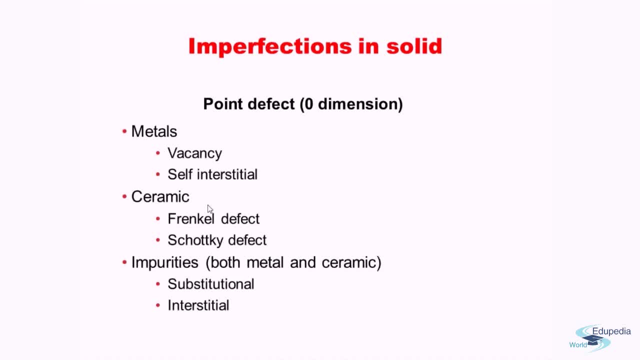 metal or ceramic atom from its initial position. So the impurity atom will displace a original atom and take its position. That is substitutional, Interstitial is. the impurity atom will go and sit at an interstitial site, It will not move. 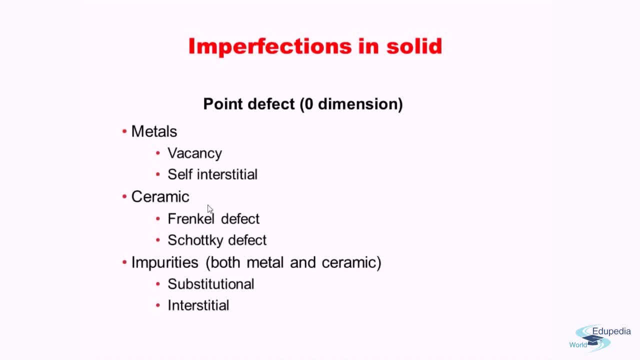 It will not displace any atom. So these all are, broadly speaking, the point defects that can be present in a solid. Now that we have an idea about the point defects, we'll see all of them in details and their importance, their significance, how they affect the properties of solid in coming lectures. 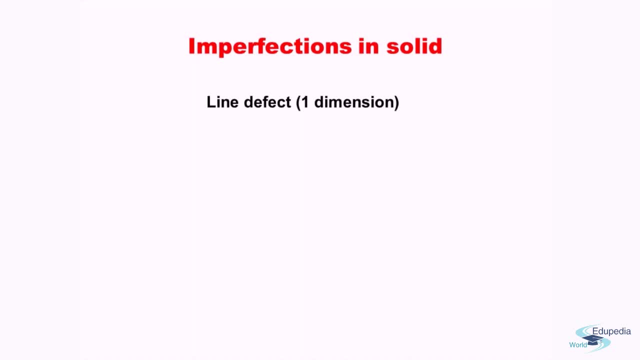 Next let us see line defect. Line defect, as the name suggests, line is a one dimension, So line defect are basically one dimensional defects. So instead of atoms missing, there will be line of atom missing or line of atom additional atoms present where there should not be right. 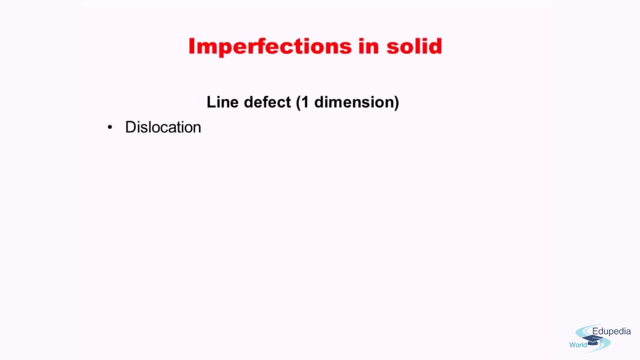 So the line defect is basically known as dislocation. Dislocation can be of two categories. It can either be a edge dislocation or it can be a screw dislocation. So the line defect is basically known as dislocation. A third category is basically a combination of edge and screw dislocation, which is known. 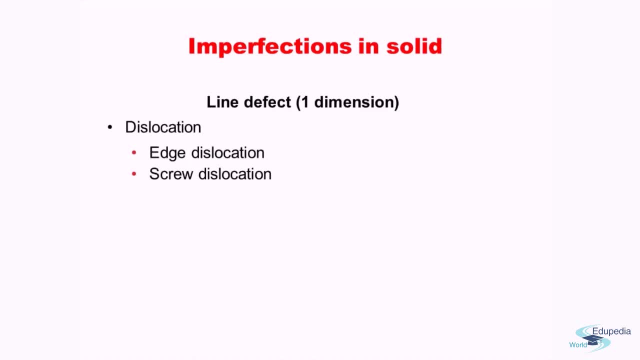 as mixed dislocation. I'm not going into the details about these things. This is a brief introduction. We'll go into the details in coming lectures. So now we know what is line defect. Next let us see what are the surface defects possible. 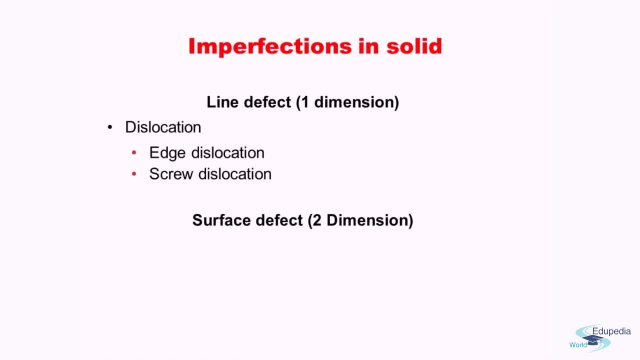 Surface defect: as the name suggests, any surface is a two dimensional thing, right? So let us see what are the surface defects possible. Surface defect: as the name suggests, any surface is a two dimensional thing, right? So a surface defect is a two dimensional defect or two dimensional imperfection in. 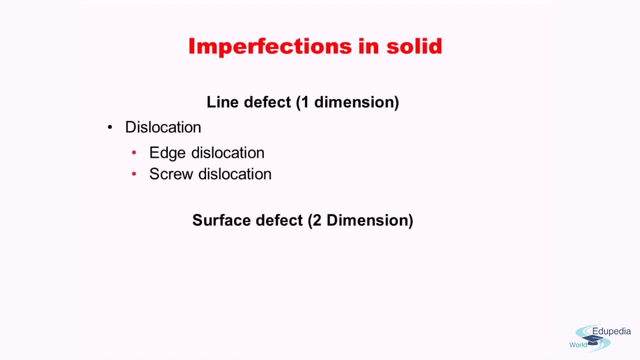 a solid. So what are the possible surface defects? Some of the possible surface defects are the external surface. right External surface is actually a discontinuity, So ideally there should not be any external surface. The atoms should keep on arranging till infinity. 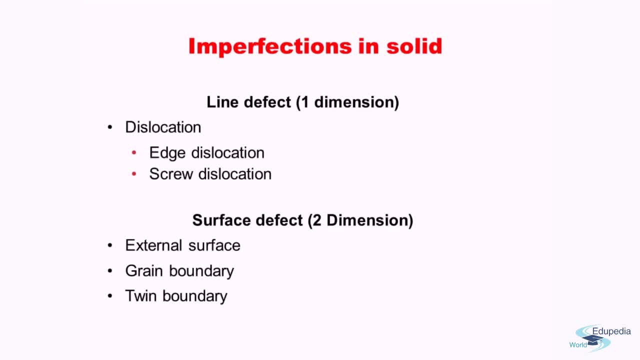 For the perfect, Perfect crystalline material to exist. But obviously that is not a practical scenario. The specimen need to end somewhere because it is a finite specimen, So it will obviously have an external surface and that is a discontinuity. thereby that is an imperfection. 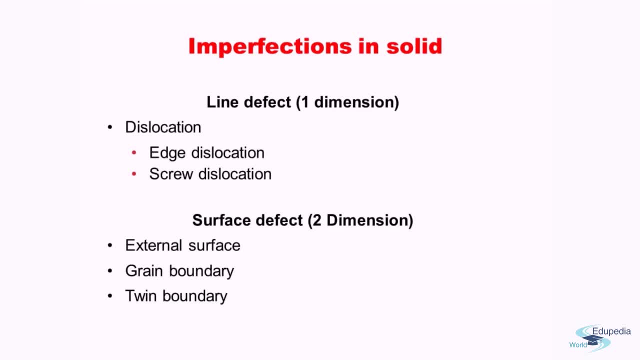 Then, secondly, we have what is known as grain boundaries. This grain boundaries comes into picture in the case of polycrystalline materials, As I have discussed in the previous lecture. polycrystalline materials are materials which have different regions of crystallinity, and each crystal region, or what is known as each 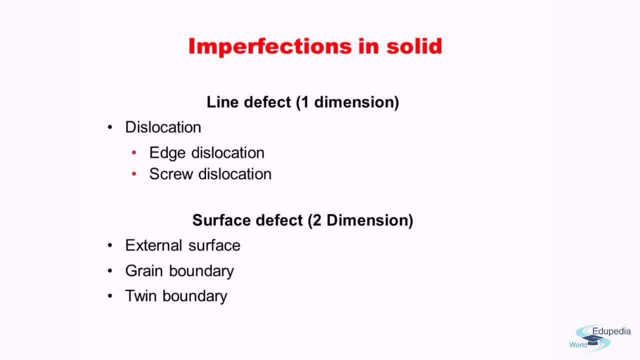 grain has a orientation mismatch with its surrounding grain. Thereby these grains have are separated by a discontinuity which is known as the grain boundary. Grain boundary being a boundary is a two dimensional defect. Then we will see something which is known as twin boundary.